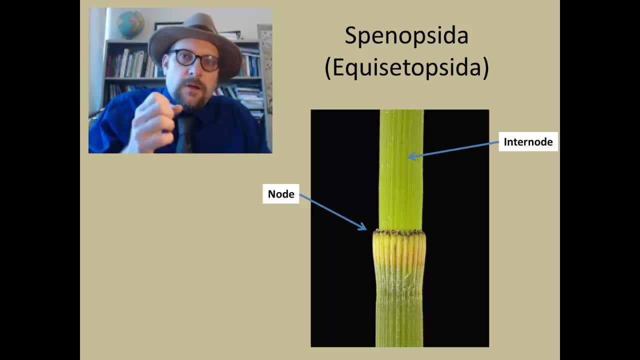 the outside, This is similar to a drinking straw. Each segment is called an inner node, with a node that fits into the next segment. This is a remarkable adaptation that allows the plant to easily break and regrow segments. This is an adaptation to herbivory, as animals that feed on horsetails would not completely. 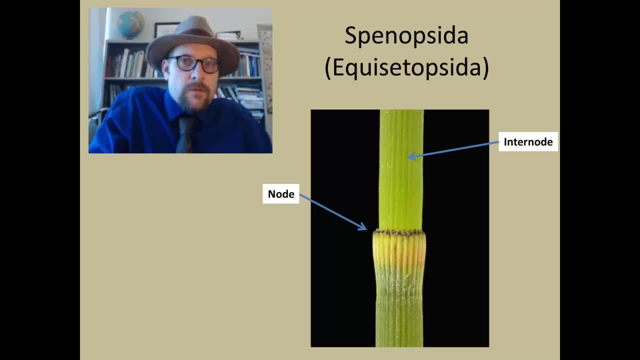 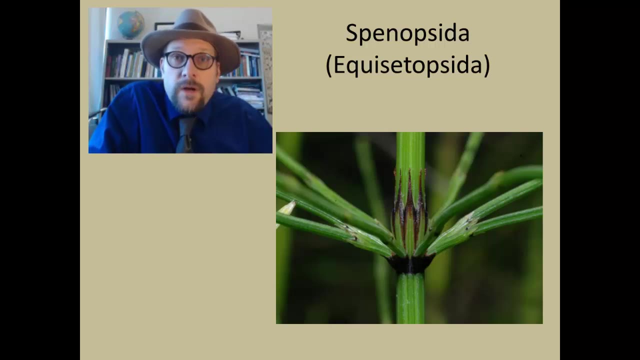 uproot and kill them, But it would allow for the upper portions to be sacrificed and later regrown after being browsed. At the end of this lecture, I will talk a little bit about what these herbivores likely were. Many modern and fossil horsetails have a ring of small leaves that extend out from the node. 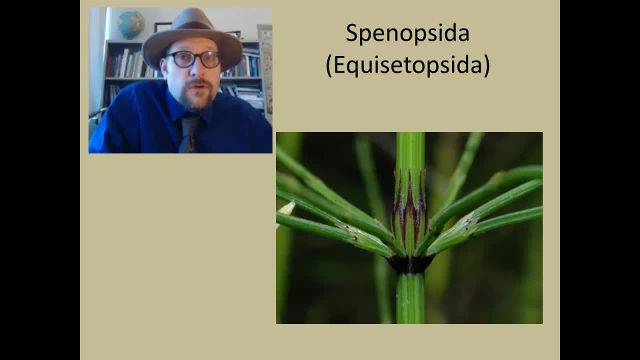 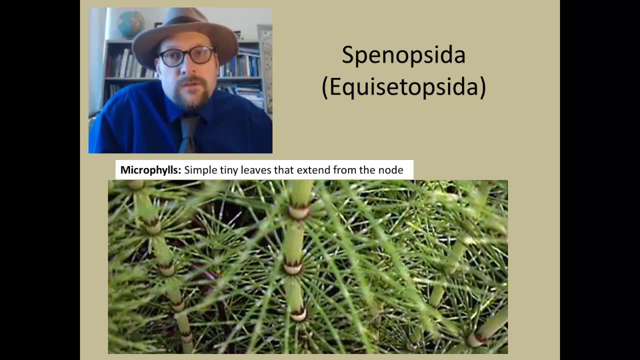 These grow in a circle around the node and provide for an additional surface area for photosynthesis. These small radial leaves are called microphylls, A word we encountered when we discussed fossil club moss. Unlike the large macrophylls that you find in ferns, horsetails have narrow, small leaves. 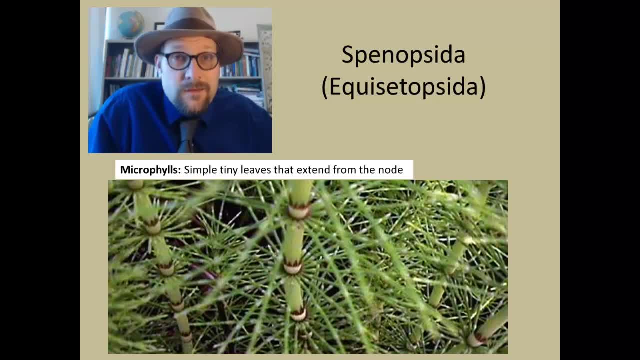 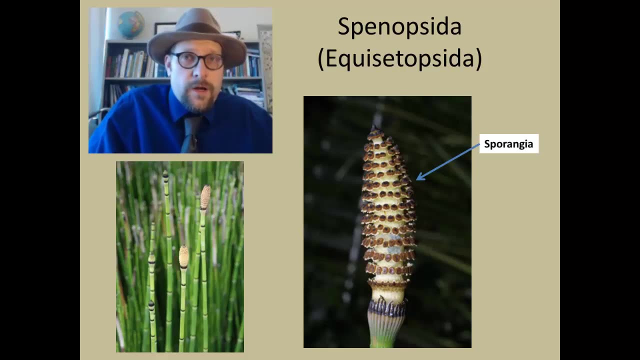 that lack the broad fronds that you see in ferns and later plants. Some horsetails in the fossil record do expand the microphylls somewhat to resemble more leafy leaves Like bryophytes, club moss and ferns. the horsetails are also spore-bearing plants. 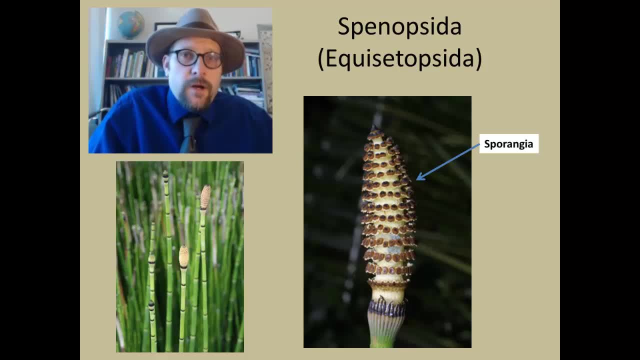 At the end of each stalk is the sporangia, a spore-bearing cone that appears during parts of the year. Unlike the spore-bearing sporangia we have previously seen, such as the capsule-like ends of primitive bryophytes and in the fossil Cooksonia, the sporangia is arranged in a spiral cluster. This cone-like sporangia are believed to have evolved from a plant that exhibited spore-bearing sporangia along the tips of leaves. These leaves have been retracted into the soil. The sporangia are believed to have evolved from a plant that exhibited spore-bearing sporangia. 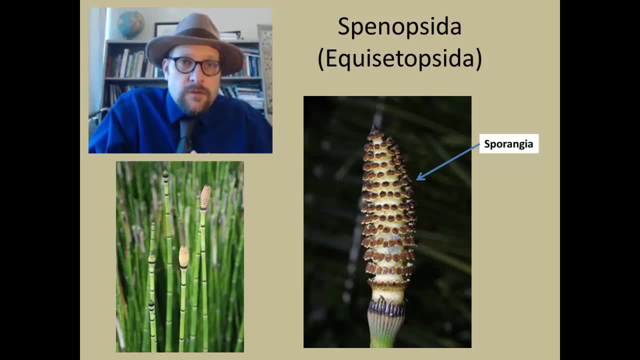 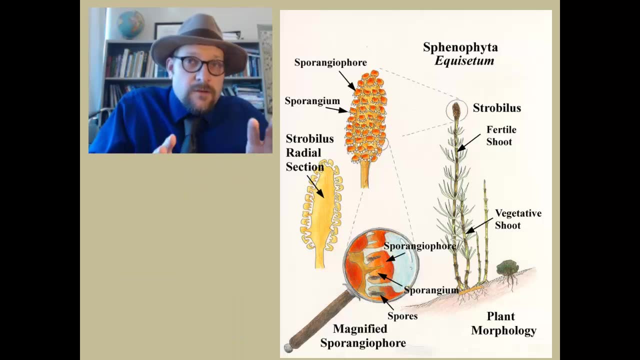 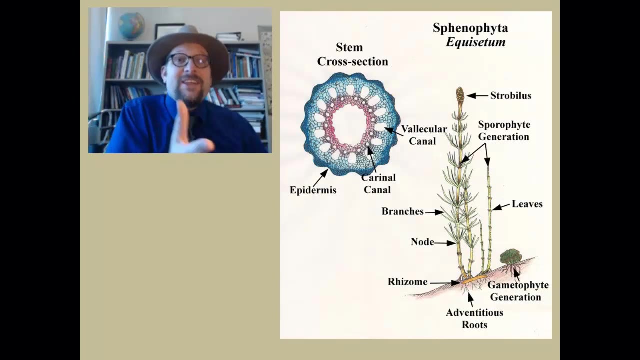 and concentrated in a cluster at the tip of the plant. The spore-bearing cone. part of the plant is called the strombolus, which contains many sporangia pores, each supporting a sporangium. the spore-bearing part of the plant. 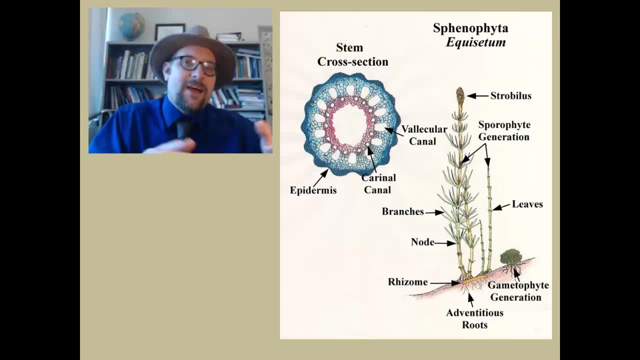 Each of the strombolus spore-bearing cones is supported by a unique vascularization. Rather than having a thick interior of coelom in the stems, the horsetails support their tall stalks with an open spore-bearing cone. 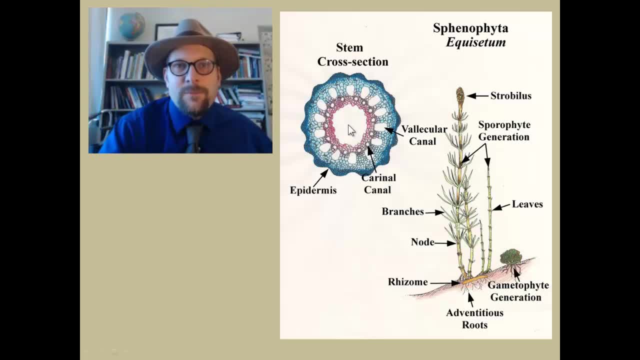 These are surrounded by smaller tubes encased with a stiff cellular wall. The ring of canals on the edge of this hollow center are called the carnal canals, while the large vallicar canals are beneath the fleshy, stiff epidermis on the outside. 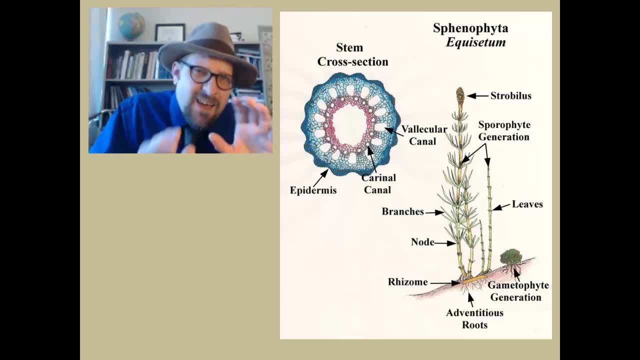 With this arrangement, the stalks are rather stiff and you would think this would not be enough to support much growth. However, using the air-filled central canal as a structural support, and with the added benefit of the reduction in weight with the air-filled center, the horsetails can get. 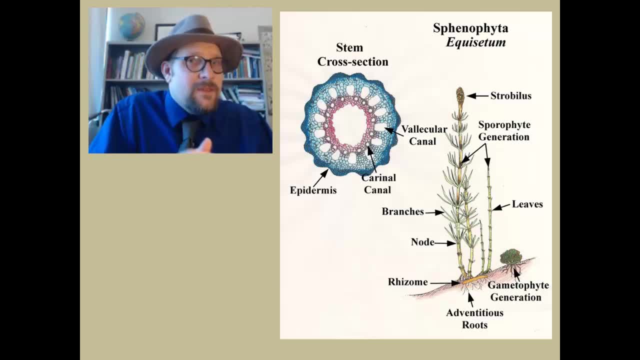 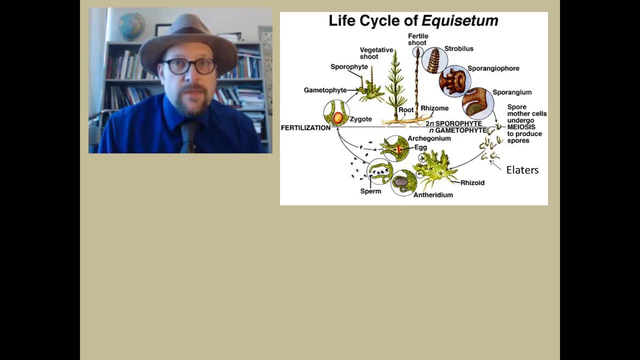 several meters high and, as we can see in the fossil record, get to be the size of large trees. Also, remember that these tall stalks are the sporophyte generation and that the small gamophyte generation still is required for the life cycle of horsetails. The life cycle of horsetails is similar to what we saw with the clansmen. The spore-bearing cone- part of the spore-bearing cone- is the spore-bearing cone. The spore-bearing cone- part of the spore-bearing cone- is the spore-bearing cone and the spore-bearing. 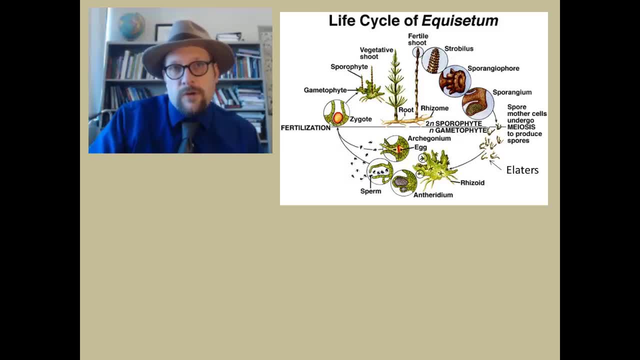 cone is the spore-bearing cone. A hidden gamophyte generation is burried in the ground and during the wet season the gamophytes produce hundreds and thousands of sperm, which swim in the water to find eggs in the archigotium. 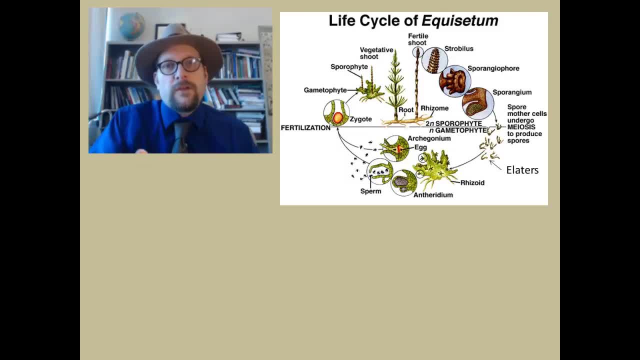 To fertilize the egg, to produce the zygote. it develops into the sporophyte generation, which is the large part of the plant that bears spores through meiosis, which then grow into the gamophytes. Now, one unique thing about modern horsetails is spores. 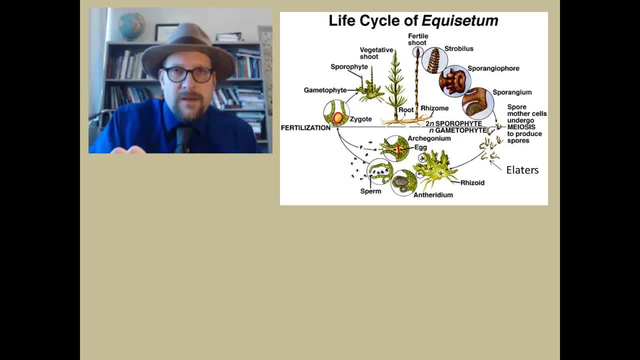 The spores exhibit elaters, which are tiny thread-like extensions off the spore membrane that extend out from the spore and help to catch air currents. When they fall in a moist environment, the elaters change, forming a sticky surface that allows the spore to stick to the moist surface. 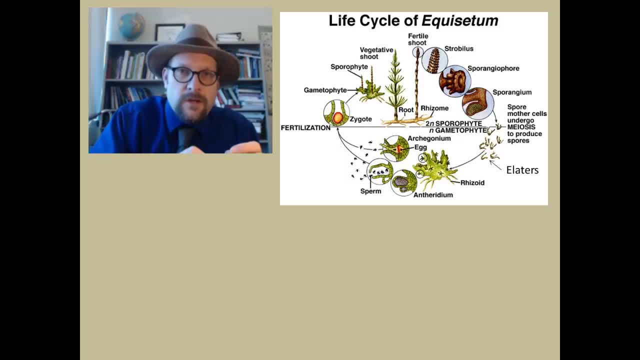 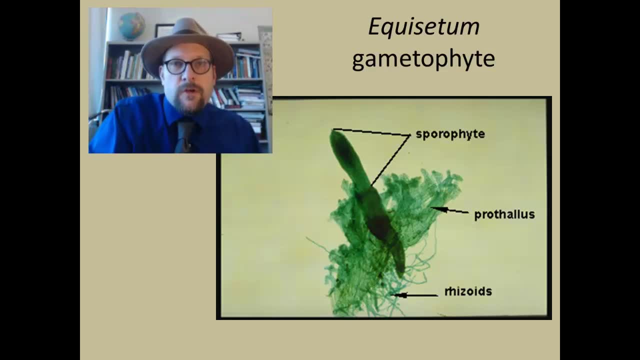 If the ground they land on is dry, the elater does not form a sticky surface and the spore is free to keep blowing down the road. So now, if we look at a typical gamiphyte generation in the wet ground, we see that it contains. 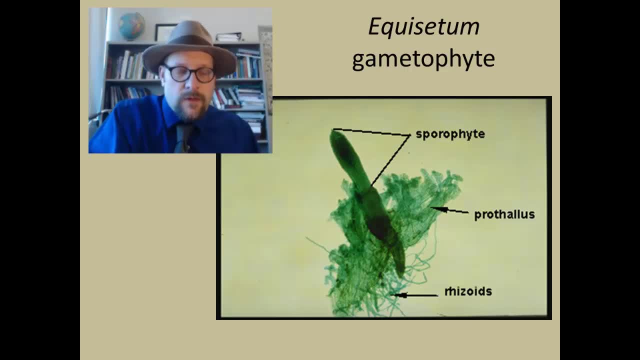 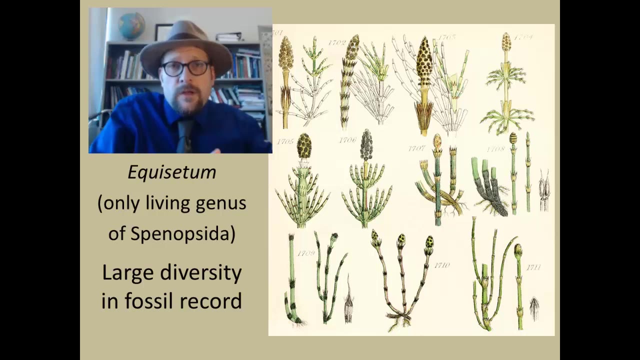 the simplest of structures, a few cells that compose the thalus, a few rhizodes that hold the plant down, and within the archegodium we have a sprouting baby sporophyte generation. Now, today, there is only one generation, The genus of horsetail Ectocetum, which is split into 25 or so species. 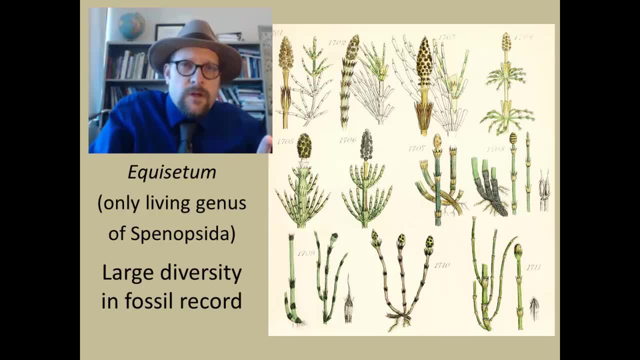 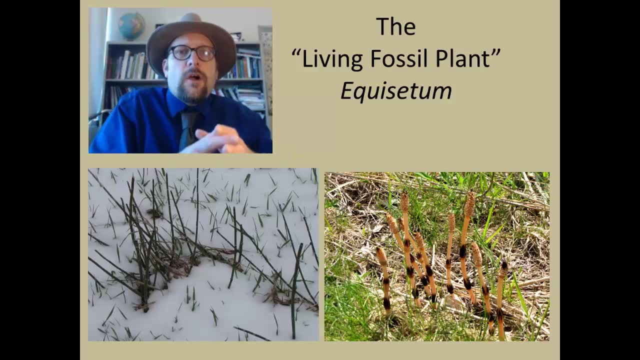 It is the relic of a much more diverse ancient group of sphinopsian plants that is only recorded in the fossil record, So we can regard Ectocetum as a living fossil plant, which at least provides us with some ideas about what the past flora may have been like. 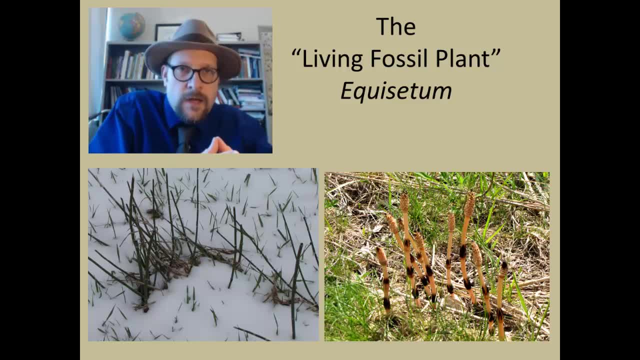 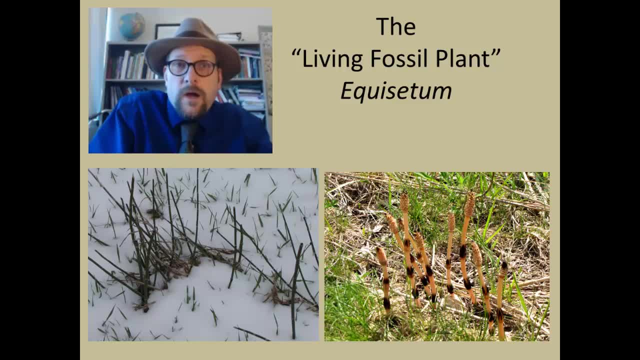 It is thought that the fossil sphinopsians may have had a similar wide range of climate tolerances and can be found in colder regions not supportive to club moss and ferns. However, modern horsetails do require a wetland or seasonally wet ground to grow well. 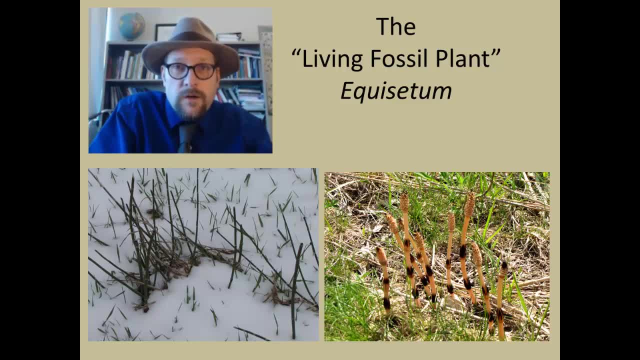 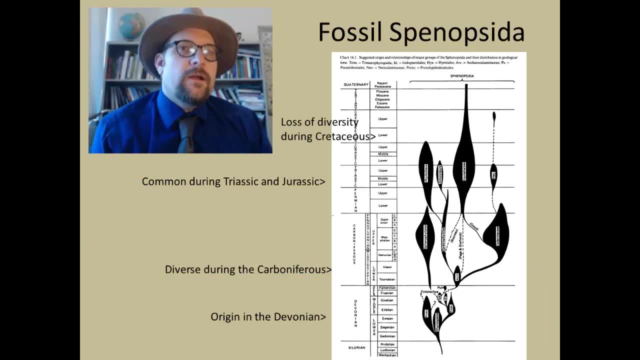 Often the stalks of horsetails can grow far from the sources of water, but they can't grow in a really dry desert environment without a local source of water. The fossil record of sphinopsians is that they can grow in a very dry desert environment. 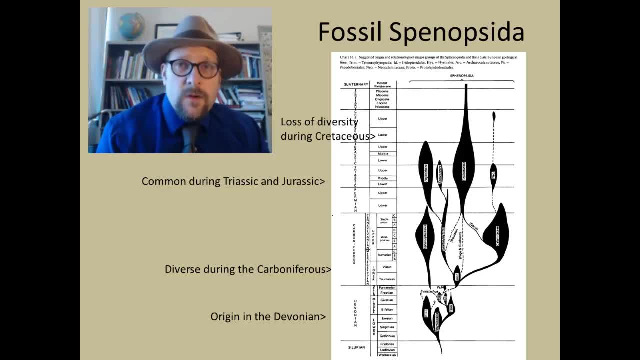 without a local source of water. The fossil record of sphinopsians is that they can grow in a really dry desert environment without a local source of water. The fossil record of sphinopsians goes all the way back to the Devonian, when they originated. 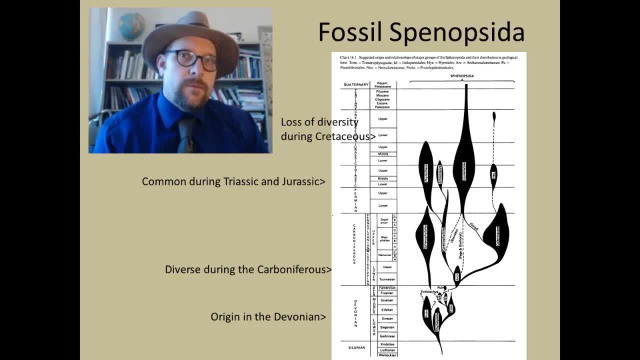 alongside the earliest vascular plants During the Carboniferous they became very diverse, including the group called the Kalmatisi, which were rather large and dominant in the Pennsylvanian During the Permian and even across into the Permian Triassic. the horsetails did rather 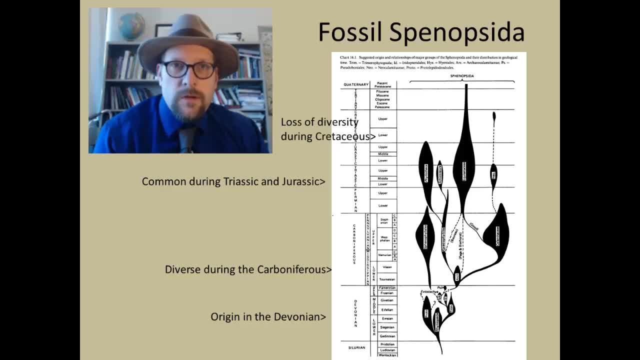 well, with Equisetians becoming the dominant group During the Triassic and Jurassic, the horsetails were wide-spinned. During the Triassic and Jurassic, the horsetails were wide-spinned. The horsetails were wide-spinned. 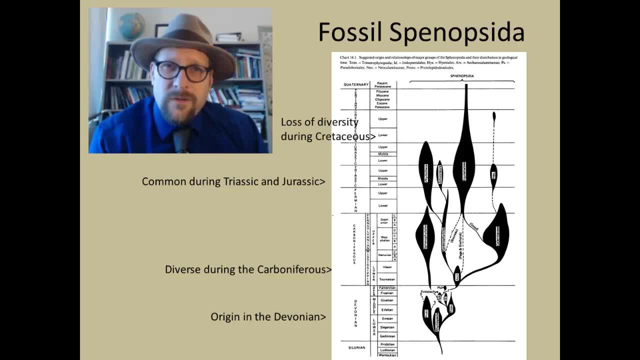 The horsetails were wide-spinned, But, as for the Cretaceous, the horsetails started losing out in diversity. This drop in diversity of the sphinopsids and horsetails during the Cretaceous might reflect the competition with modern angiosperms, the origin of today's grasses, which could 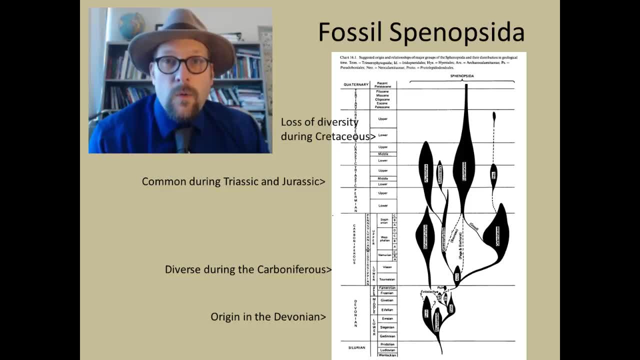 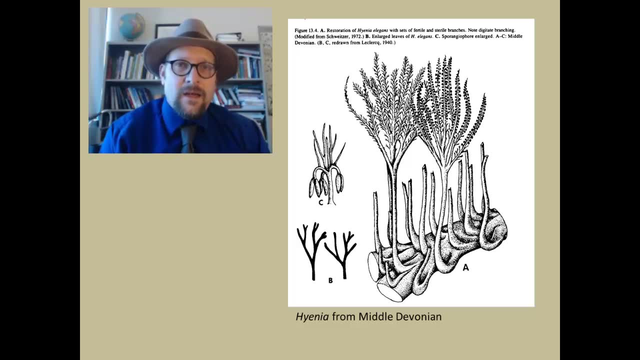 grow in dry environments and may have out-competed the grass-like horsetails. Alright, so let's dive into the fossil record and look at some of these fossil sphinopsians. This is Hyena, A fossil from the Middle Devonian. this Phineopsidant plant exhibits many shoots that extend from: 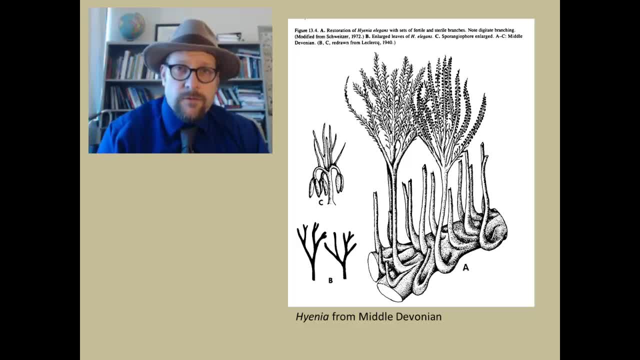 a central basal stalk with fronds of microfil leaves with clusters of sporangia pores. This plant does not resemble modern horsetails but exhibits features that make it closer related to the group, possibly a transitional fossil. Not much is known about the vascular tissues of this plant, which might help to determine. 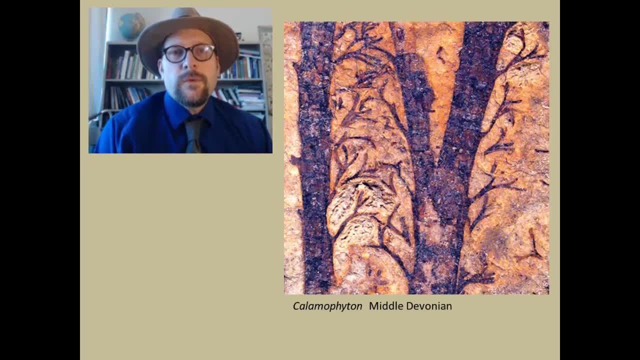 its relationship to later groups. The first fossil that really shows a more modern horsetail condition is the Middle Devonian Clamatophyton, which appears to have had a more segmented stalk with primitive node internodes as well as small microfills that extended from a central stalk or stem. 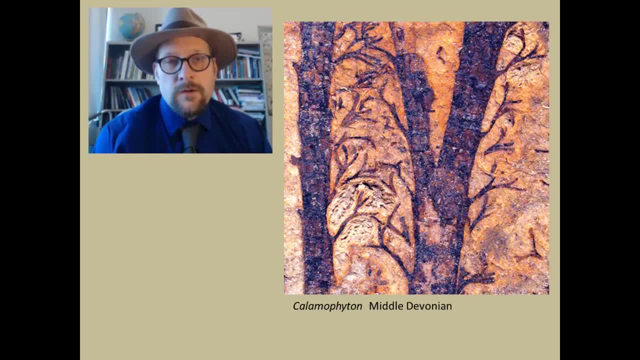 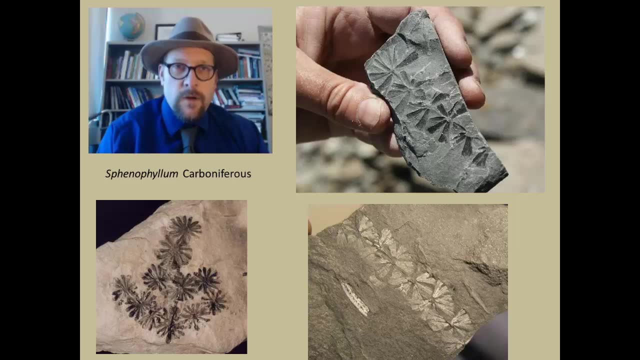 These rings of microfills are not necessarily symmetrical like in modern horsetails. One of the more common Phineopsidant fossils found in the Carboniferous is the genus Spheniophyllum, which exhibits larger microfills projecting from the nodes symmetrically in rings. 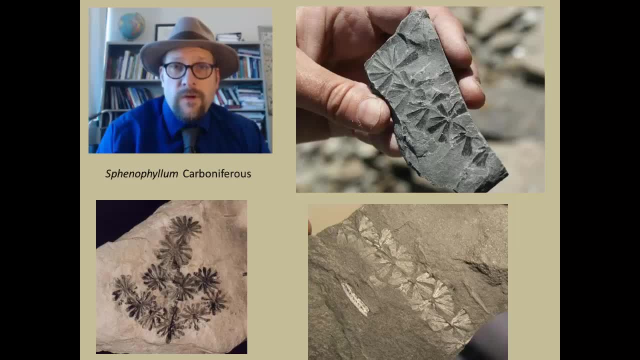 There are either 6 or 9 leaves to each ring. Spheniophyllum is believed to grow like a bush, with sprouting stalks extending from a central stalk. although fossils showing this arrangement may be pure conjecture, The leaves are rather broad for a Phineopsidant in Spheniophyllum. 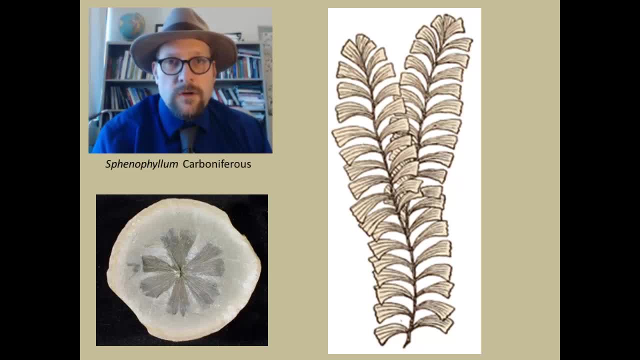 The study of the vascular stems shows that they lack the hollow center and rather have an array of canals through the stalk. However, they do have clusters of secondary xylem along the stems, indicating possibly some segmentation of the stalks. In some ways, the central stalks resemble the vascularization found in ferns. 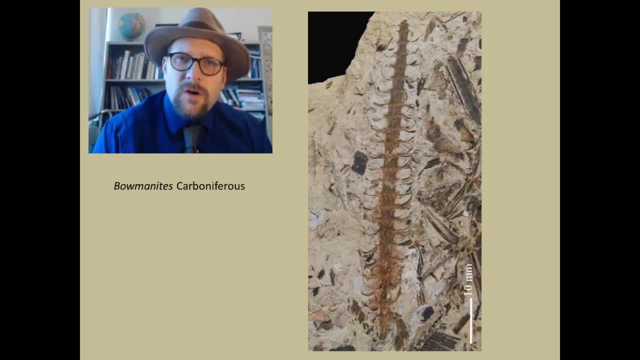 The related Bo Matis, also from the Carboniferous, more closely resembles a modern horsetail with its clusters of microfills. The similarity between Spheniophyllum and Bo Matis is most commonly found in the spore-bearing cones, as both fossils have a more complex 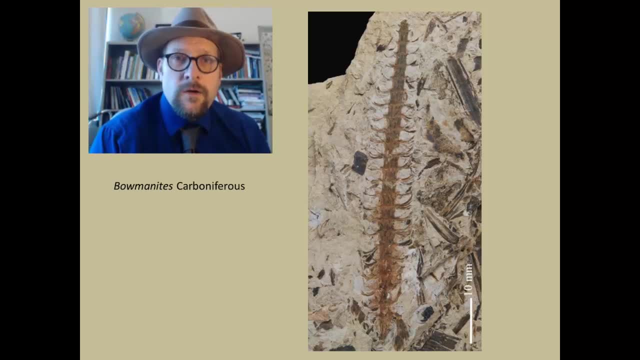 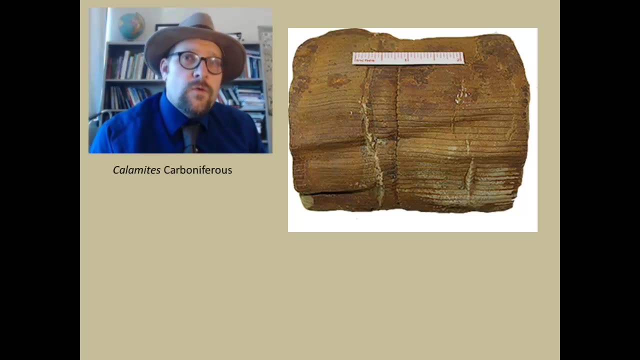 strombolus, with multiple sporangia arranged in a whirling pattern at the top of the stalks. The other major group of fossil Phineopsids in the Carboniferous are the group represented by the giant Kalmytes. This is a massively large fossil log. 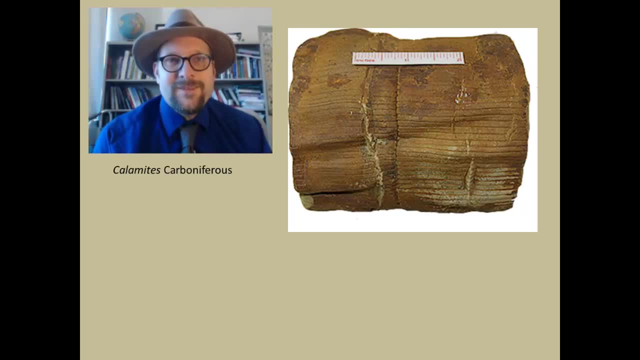 It's a small portion of a once-giant horsetail that lived during this time. Kalymates is a tree-like fossil from the Carboniferous and they grew into large tree-like plants. Their large size often excludes the group from the same group as modern horsetails, but 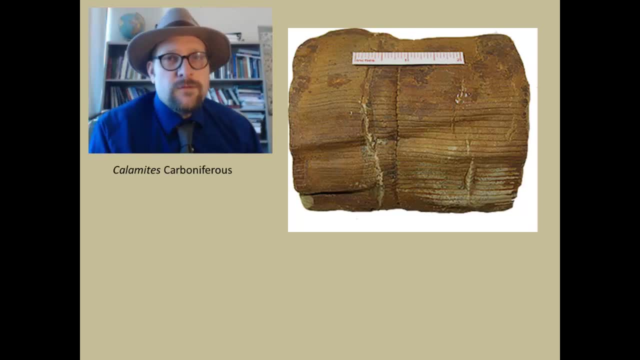 most paleobotanists group, the two together, As you can see from this fossil. the outer surface of the fossil sort of resembles modern horsetail stalks in its growth pattern. In fact, this is the first time we've seen such a group in our history. 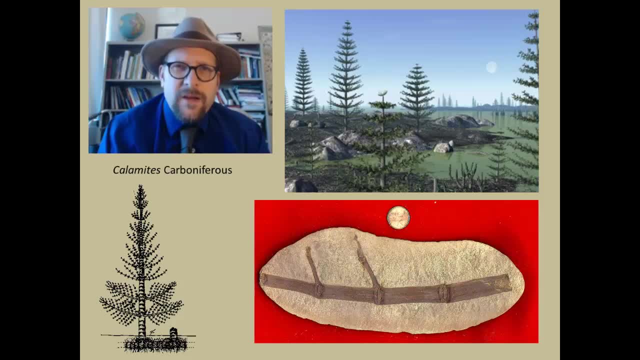 In fact, this is the first time we've seen such a group in our history. In some areas, Kalymates would have been the major tree in the Carboniferous forest, growing many meters in height Like modern horsetails. the branches would actually be segmenting off of the nodes in 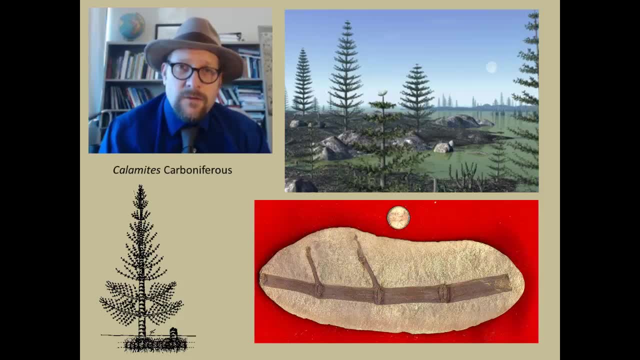 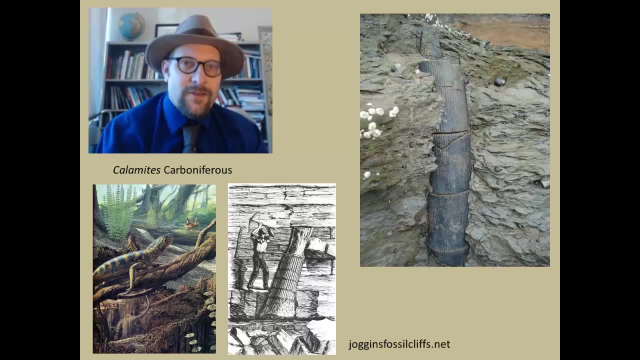 a spiral or whirl from the central trunk and from these there would be secondary branches that would also extend out. The tree would be hollow on the inside. In Nova Scotia along the Joggings Cliffs are large hollow logs of Kalymates and some 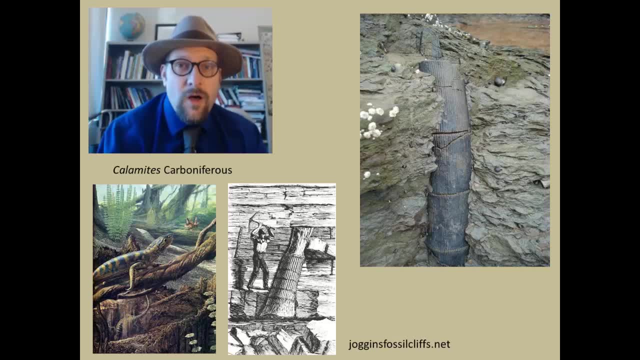 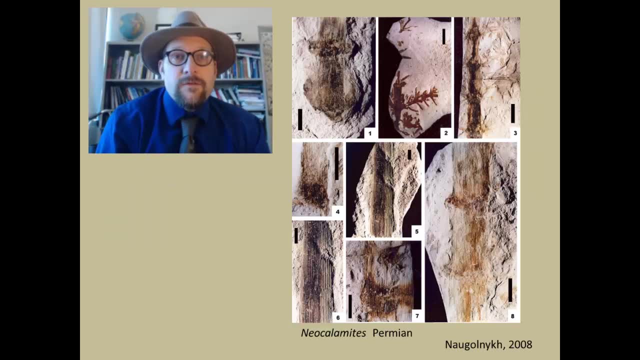 of them are preserved: amazing fossils of early reptiles which crawled into these upright hollow trunks and then were trapped and failed to escape. The fossil record of these Kalymite-like fossils extends into the Permian, where the genus Neoclamatis is found during the early Permian. 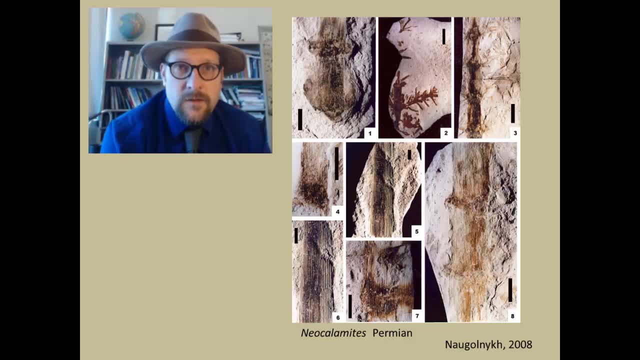 Some paleontologists have suggested that Neoclamatis is a smaller form of its ancestor, a transitional fossil between the large Kalymateses tree-like horsetails with the modern horsetails we have today. However, not everyone agrees with this assessment. 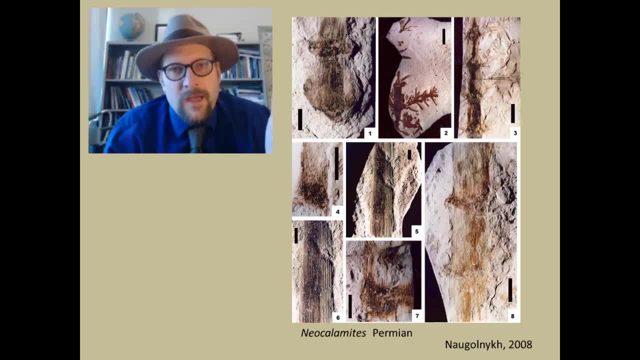 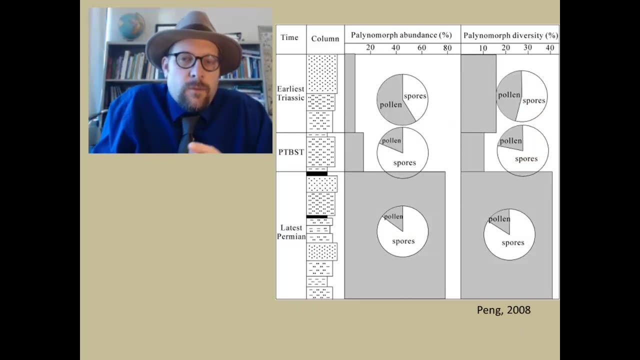 But it is strange to think about, however, that as you step over modern horsetails, there is this possibility that these simple plants today that you just ignore were once a major part of the vast forests of the Carboniferous. Another interesting thing is what happens to the horsetails. 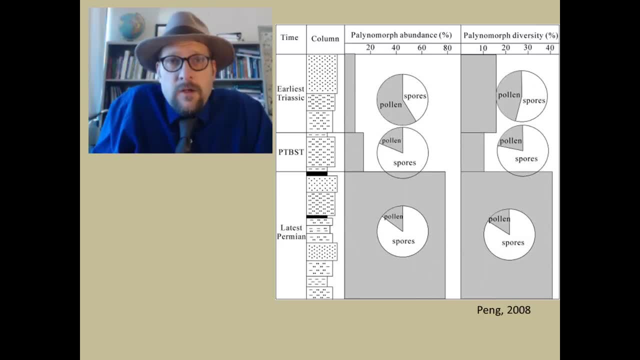 Chinese scientists have been looking at the changes- that are preserved- in the number and diversity of spores in pollen. The spores are produced by plants like ferns, club moss and horsetails, which require a wet environment to grow into gamophytes, while pollen producing plants don't have to have. 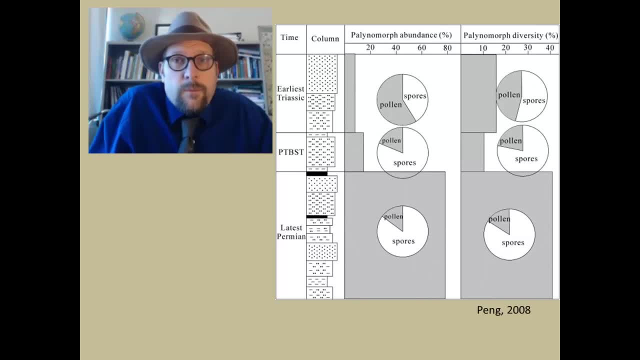 the wet requirements. Interestingly, the pattern at the Permian-Triassic boundary in China shows a step-by-step pattern in the amount of pollen to spores, such that there is an initial drop in the floral diversity across the boundary, with a period of time where the spores are still the most abundant. 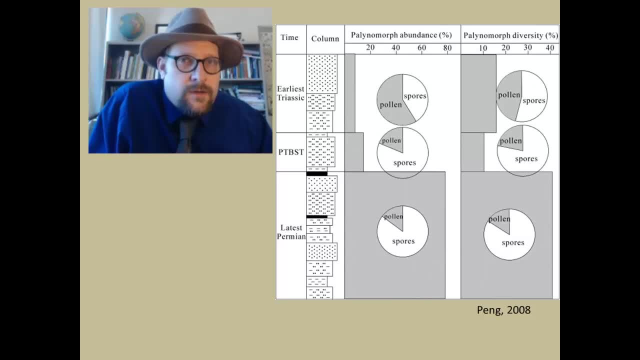 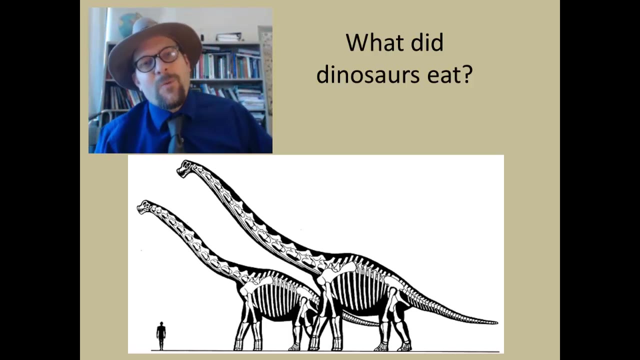 but followed later by an increased proportion of pollen in the sediments. This indicates that there was a long-lasting dry climate in which the spore-bearing plants became less and less abundant. One last interesting question: we can look at What. What? 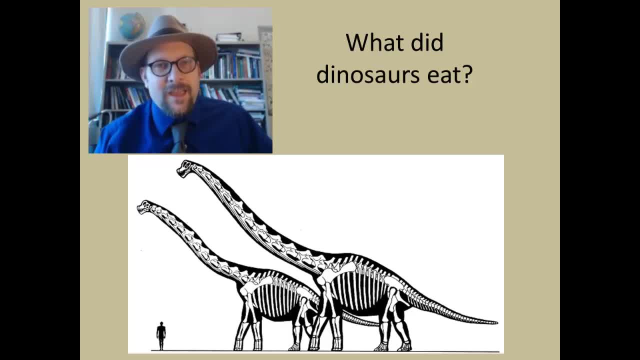 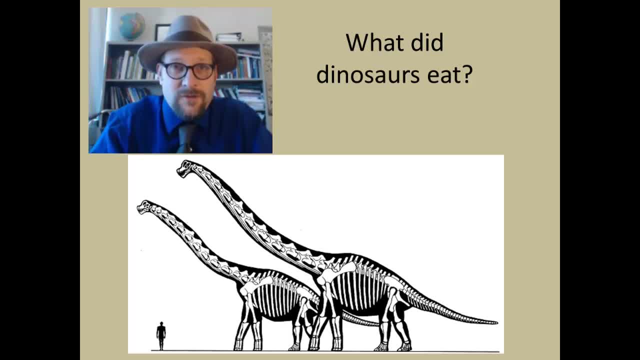 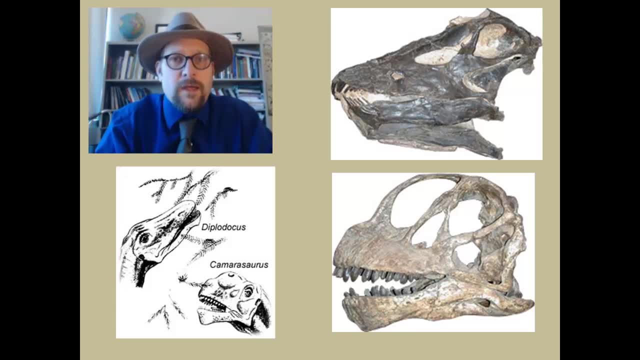 Hence all of the Jurassic fossil plants belong to just a handful of groups. What? Both of these big sauropod dinosaurs are also very blunt and peg-like and unlike the teeth found in many Cretaceous dinosaurs, which had dental batteries for grinding teeth and 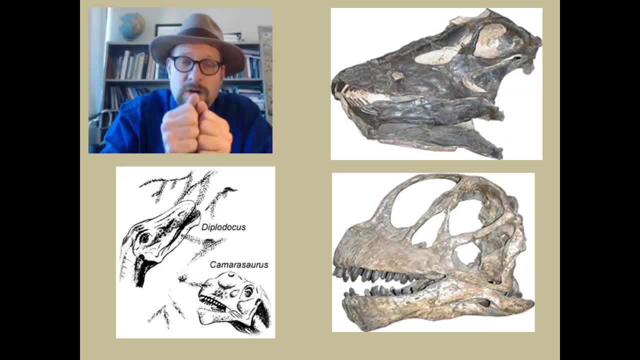 of course, feeding. that we see in mammals today which eat grass, which grind and chew their food. these giant dinosaurs had peg-like sort of plucking, like teeth, and they may have used their stomachs to do a lot of the digestion, but they were using these teeth. 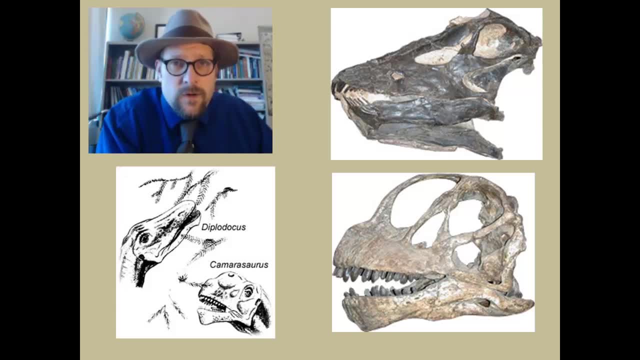 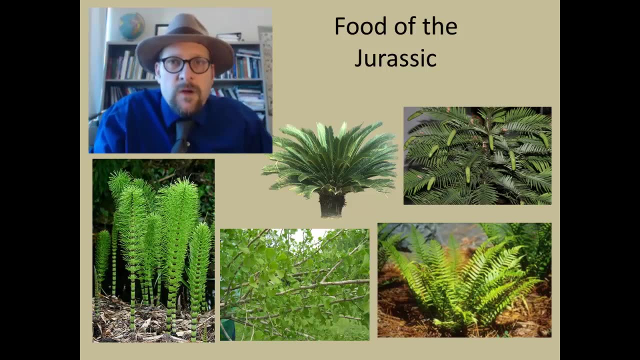 really for plucking whatever plants that they were eating. These are the types of plants that are available to these giant sauropods to eat during the Jurassic. We have really tough cycads here, not very nutritious. We have conifers. these would be like the pine trees, really tough needles. 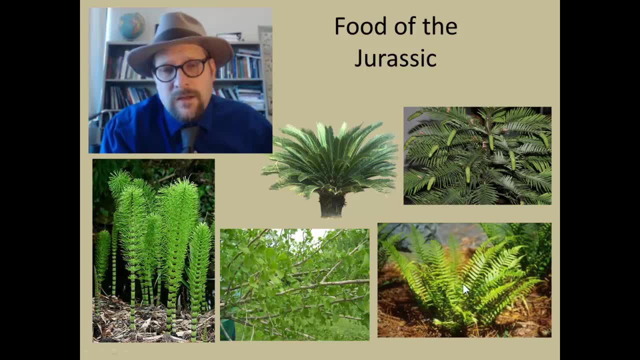 We have ferns, and many ferns are poisonous. they can concentrate poisons, things like arsenic, in their leaves. Then we have the ginkgos, which are somewhat edible, and they have fruits- they'll look at later on nuts- and then we have the horsetails. 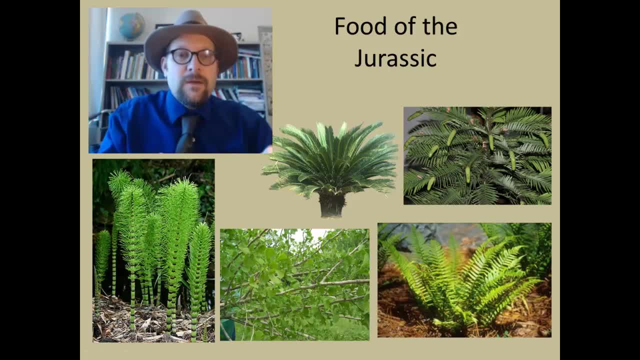 Scientists have looked at all of these plants that are living today, and they analyzed the amount of nutrition each of these plants provide, and they found that the horsetails provide the most amount of nutrition, and so the horsetails might have been the most readily available. 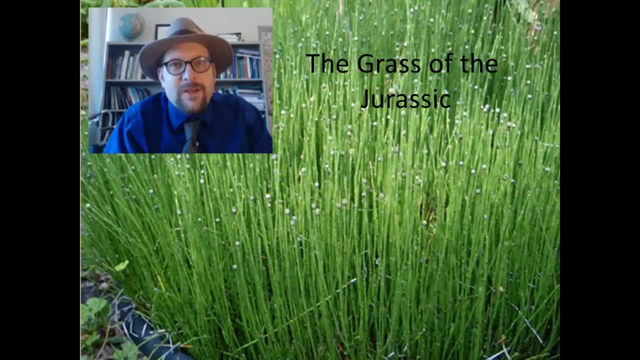 food for these dinosaurs. So what are these dinosaurs? During the Jurassic, horsetails were likely the major food source for these giant dinosaurs, and they would come along and they could pluck off the various portions of these plants and eat them. 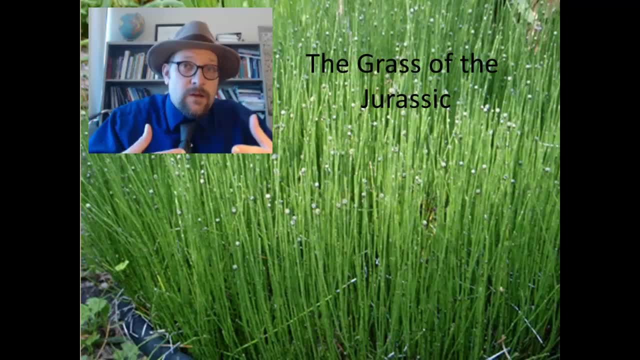 Dinosaurs would be browsing horsetails across the wetlands, which could quickly regrow to support these massively large creatures that would need a constant source of food. The horsetail is basically the Mesozoic equivalent of the modern grasses, But today feed the large herbivores that we have with us in the modern realm. 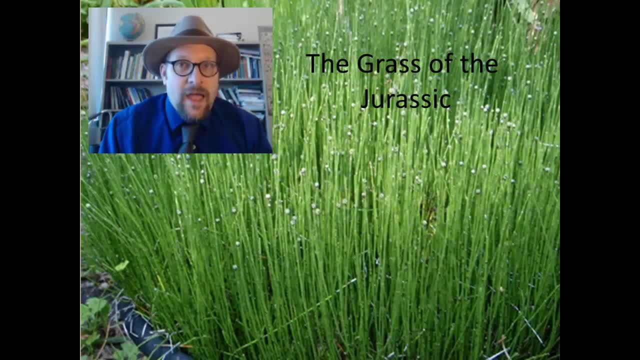 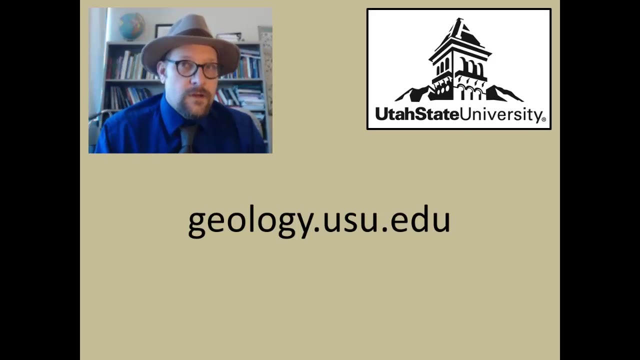 I hope you enjoyed this lecture on the fossil record of horsetails and that the next time you see a horsetail growing you'll think of dinosaur food and giant hollow trees of the past. Thanks for watching. If you are interested in taking a course at Utah State University in Geology, take a look. 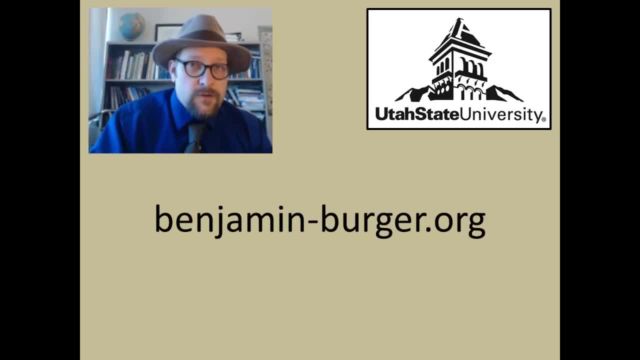